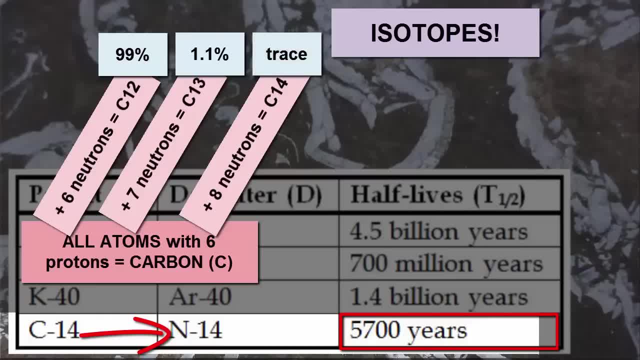 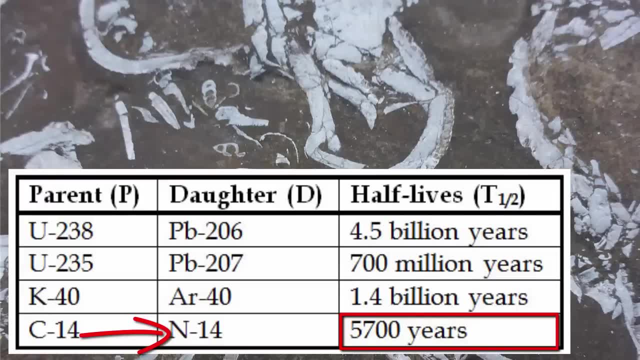 and some trace amounts of the radioactive carbon-14 isotopes. What makes carbon-14 and nitrogen-14 a very good isotope pair is that most substances that contain carbon in a structure, such as shells made of calcium carbonate, do not also have nitrogen in them. 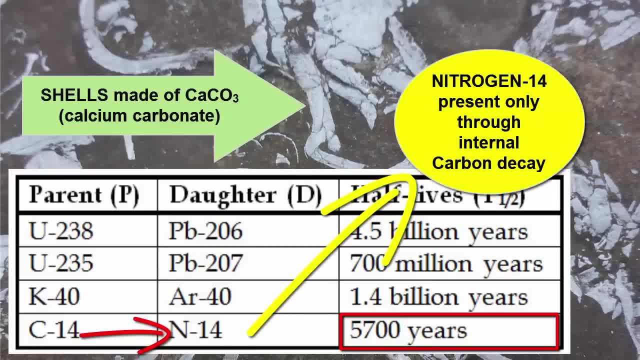 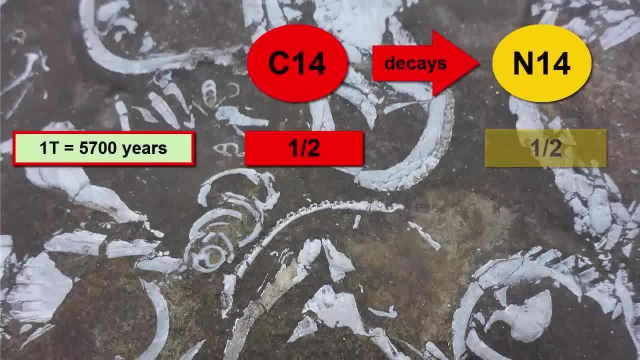 So any nitrogen-14 we see in the material will have come from the decay process For carbon-14, every 5,700 years half of the original carbon-14 has decayed to nitrogen-14. After one half-life, assuming there was no nitrogen-14 to begin with in a rock sample. 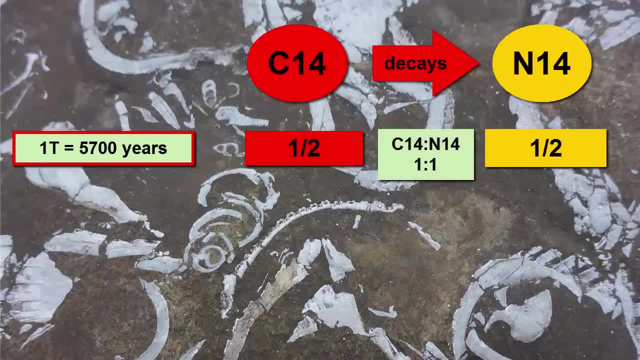 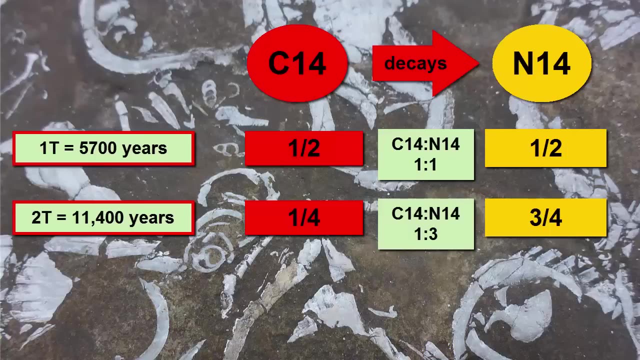 the ratio of the two should be 1 to 1, equal After two half-lives. the half that remained of parent after the first half-life is now halved again. Half of a half is a quarter. The remaining three quarters is daughter and the ratio of parent to daughter is 1 to 3.. 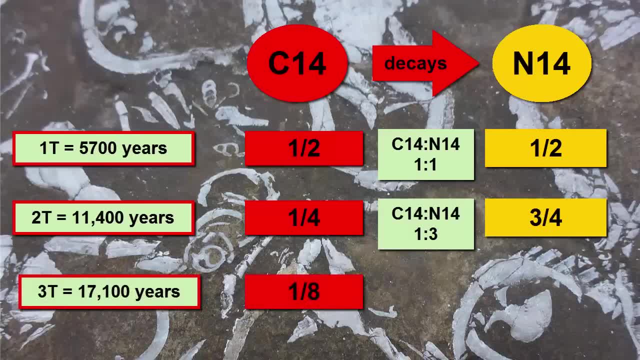 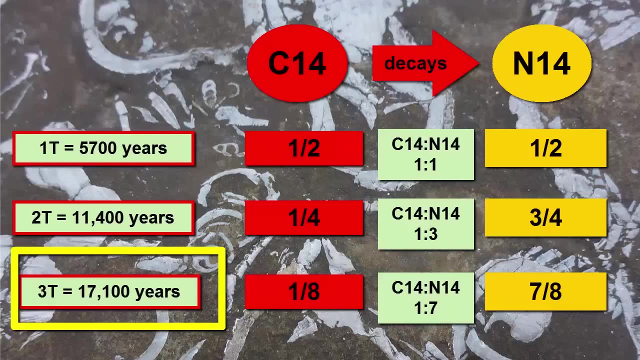 Another half-life and we halve the quarter. There's now one-eighth parent and seven-eighths daughter, And the ratio is 1 to 7, and so on. At this point, three half-lives have passed and the time is 5,700 times 3, or 17,100 years. 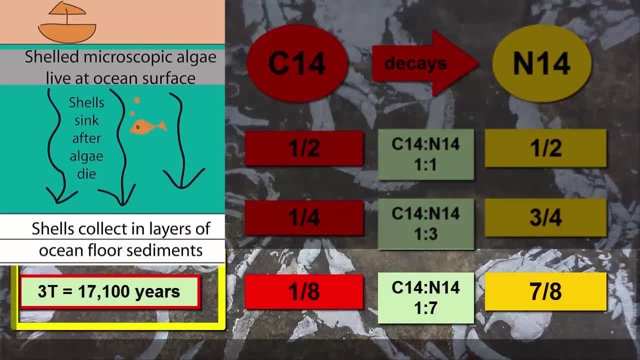 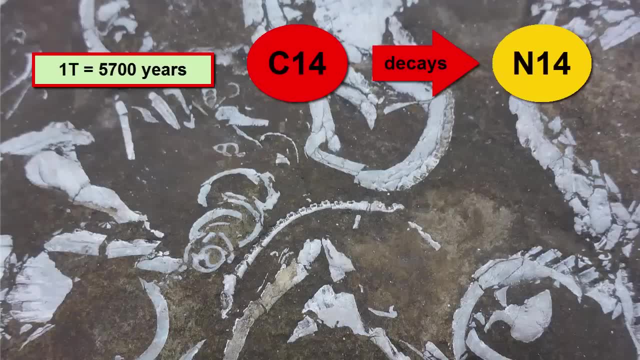 A shell that was buried 17,100 years ago would have a carbon-14-nitrogen-14 ratio of 1 to 7.. If we are trying to use the carbon-14-nitrogen-14 radioactive decay pair to date, a rock that's 100 million years old. 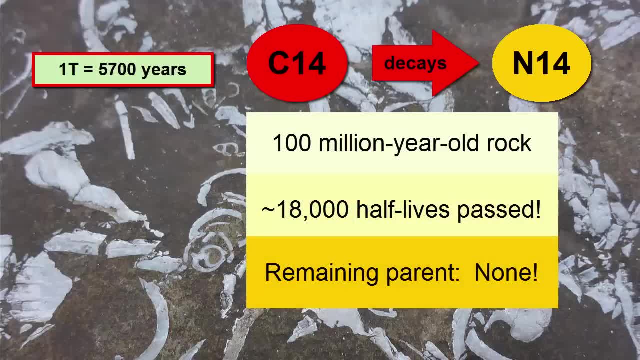 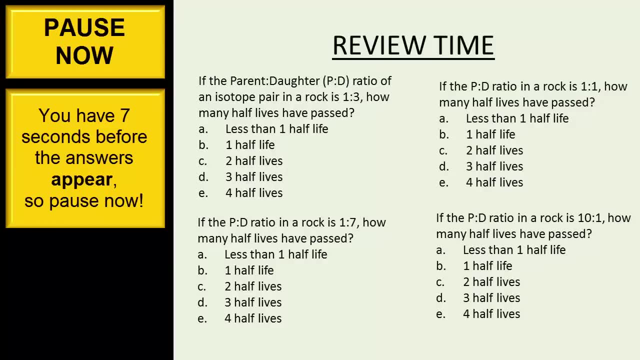 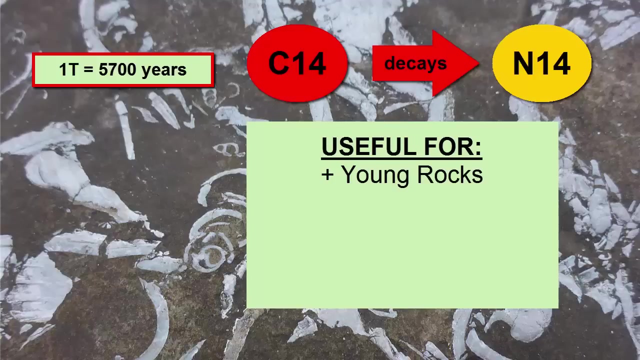 there likely will not be enough pairs. There's only one parent left to measure, and that would not be a good choice. Pause now. In addition to the carbon-14-nitrogen-14 pair being useful only for relatively young rocks, this pair is also useful only if there is carbon in the rock. 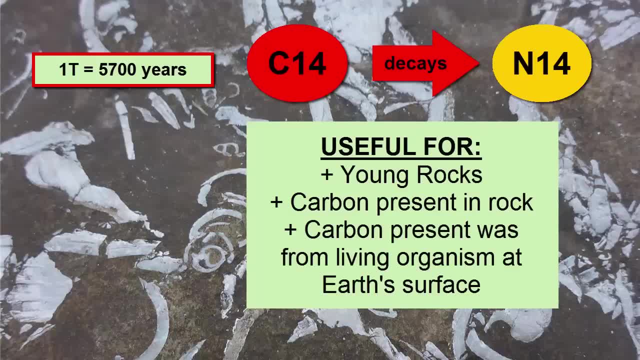 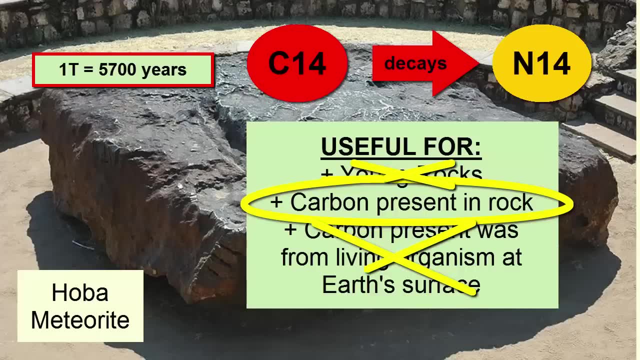 and specifically carbon that was present in a living organism at some point on Earth's surface. While one-half of all meteorites do contain some carbon, they fail on the other two requirements, and so we need to identify another radioactive decay pair to date meteorites. 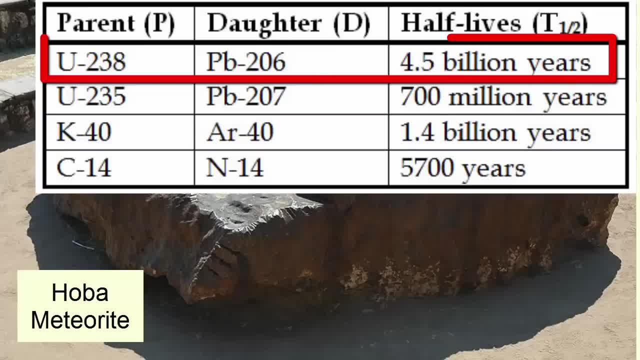 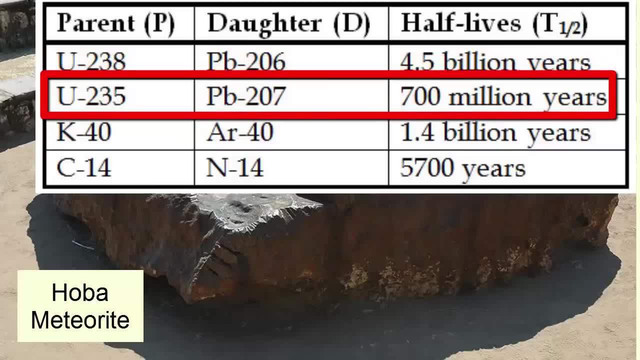 Fortunately, there are a number of other pairs, such as uranium-238,, which decays to lead-206 and has a half-life of 4.5 billion years. Uranium-235,, which decays to lead-207 and has a half-life of 700 million years. 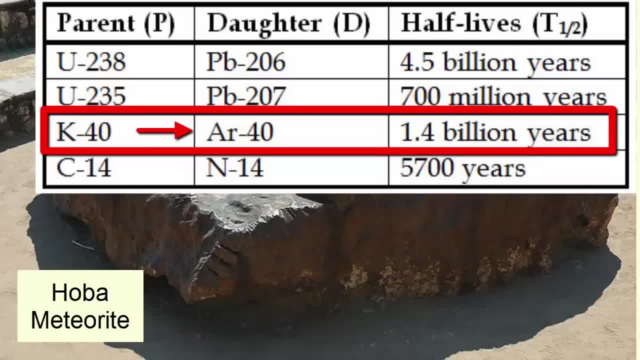 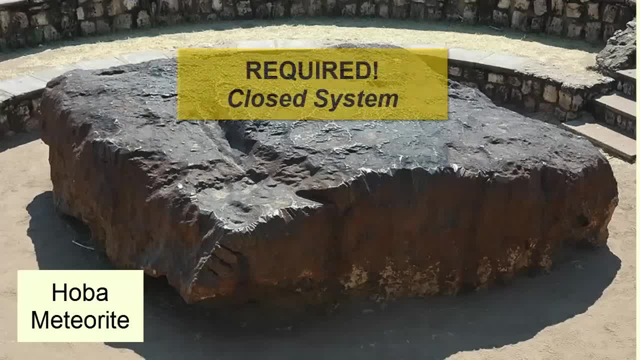 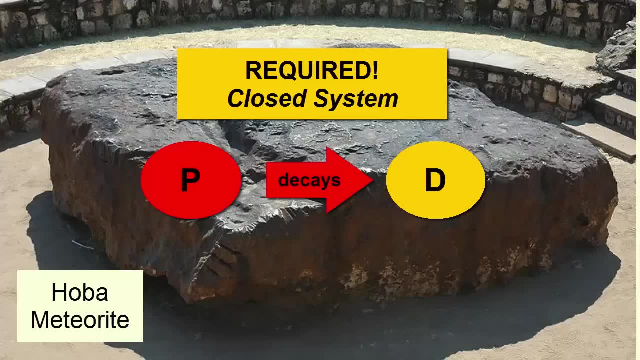 Potassium-40,, which decays to argon-40 and has a half-life of 1.4 billion years. Second step: we need to ensure the rock or shell or bone fragment has remained a closed system While parent decays into daughter. there must be no migration of parent or daughter isotopes into or out of the rock. 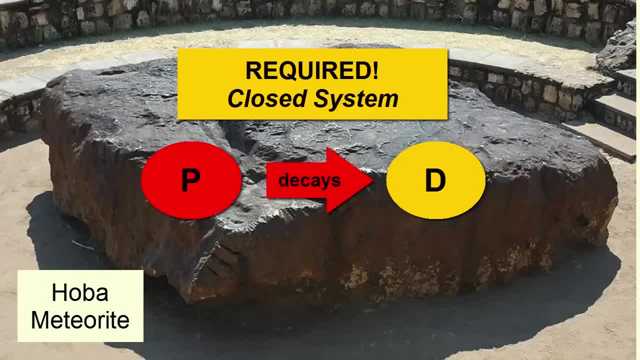 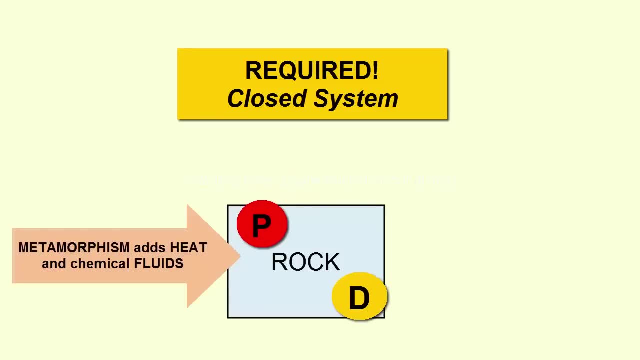 Otherwise, the ratios we see do not reflect decay over the lifetime of the rock. For example, if a rock has undergone extensive metamorphism at high heats, atoms become mobile within the rock and can migrate in and out. Similarly, if a rock undergoes chemical weathering on its surface, 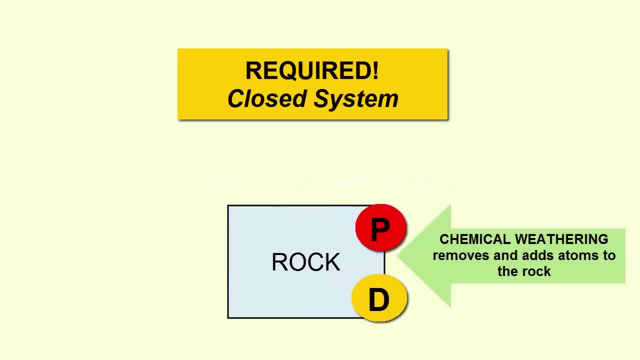 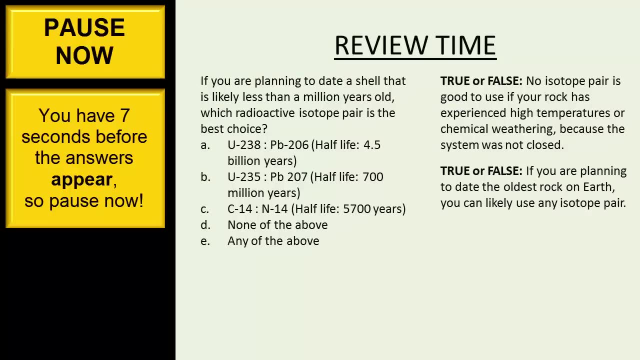 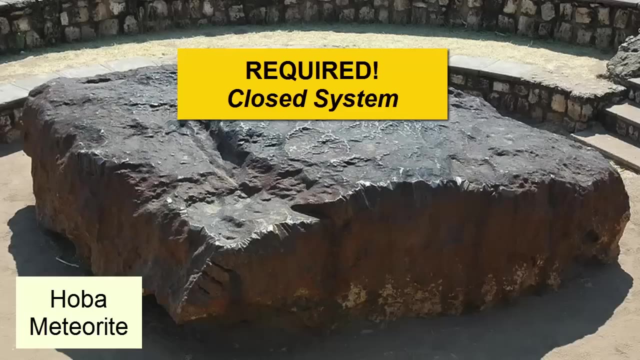 minerals can break down and atoms can migrate in and out. So how do we date a meteorite? First we ensure it was a closed system By picking a good sample without any weathering or evidence of melting. Then we place a sample of it in a mass spectrometer. 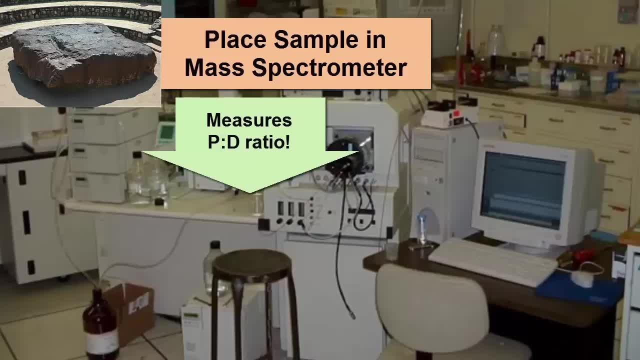 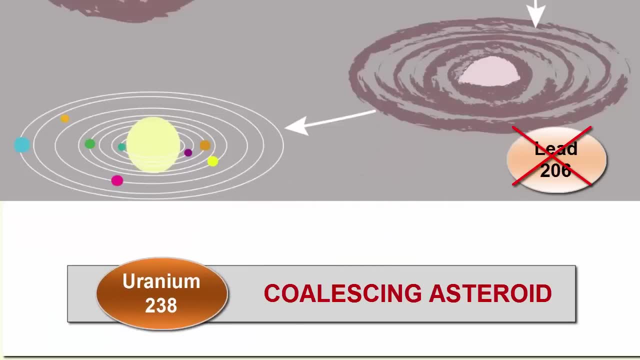 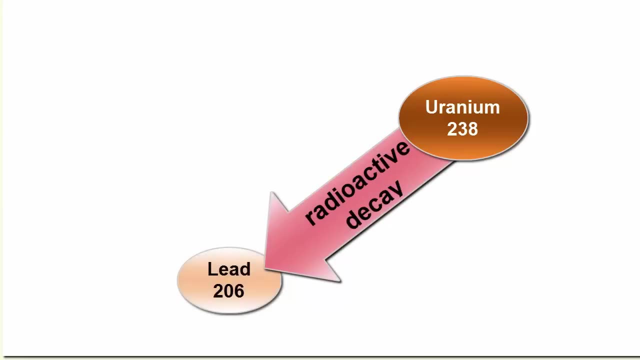 to measure the ratio of the particular radioactive decay pair we're studying, In this case uranium-238 and lead-206.. When asteroids first coalesce, they contain plenty of uranium-238, but no lead-206. The only way to produce lead-206 is as a radioactive decay daughter product of uranium-238. 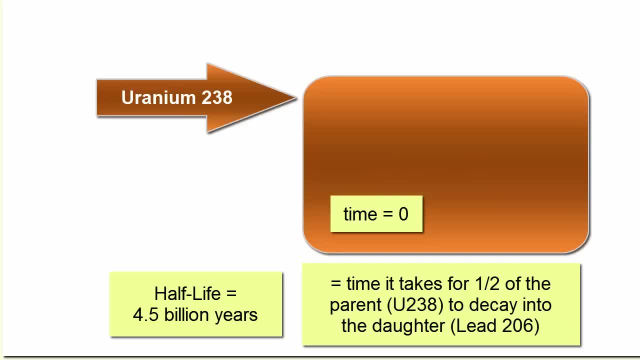 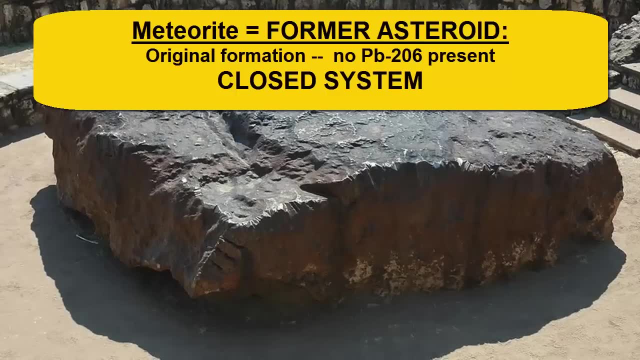 Every 4.5 billion years, one half of uranium-238 will decay into lead-206.. So if we open a closed system asteroid that formed 4.6 billion years ago with no lead-206 at that time and no loss or gain from or to the outside world since, 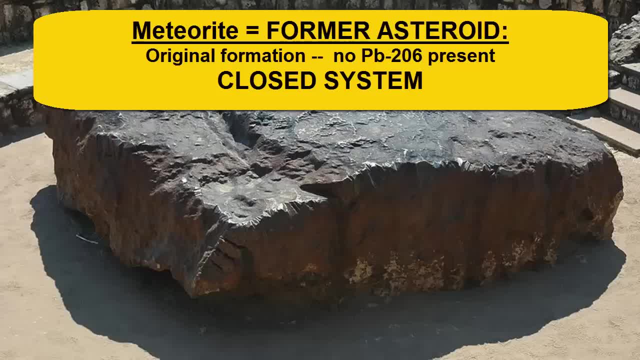 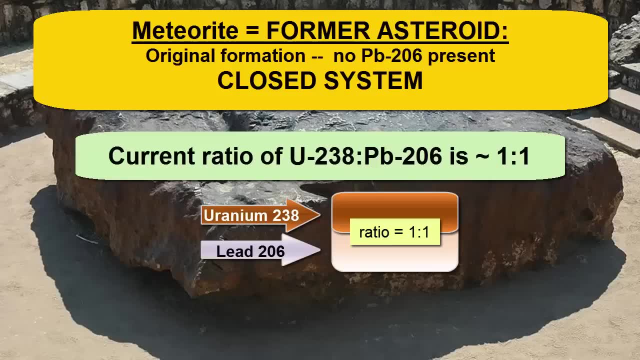 we can use the ratio of the parent and daughter within to determine how long decay has been happening or how old the meteorite is. And what do we find? Almost exactly equal amounts of uranium-238 to lead-206.. That ratio of 1 to 1 is possible only if exactly one half-life has passed. 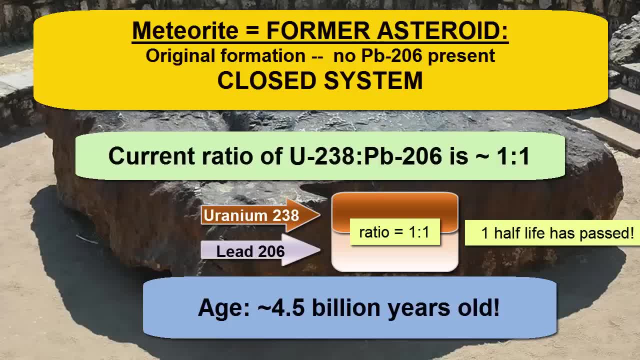 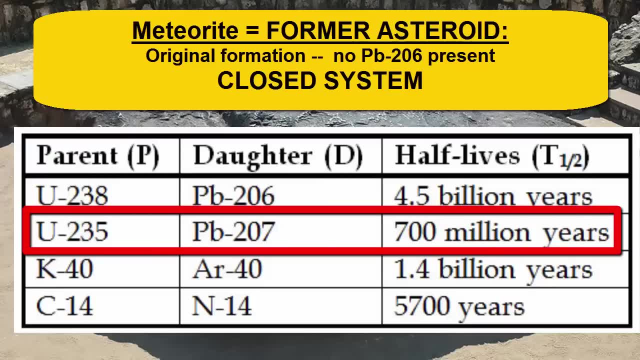 The meteorite formed about 4.5 billion years ago. Of course, in the lab we get a lot more precise. What if we used uranium-235 and lead-207 to date the same meteorite? What would we find as our ratio? 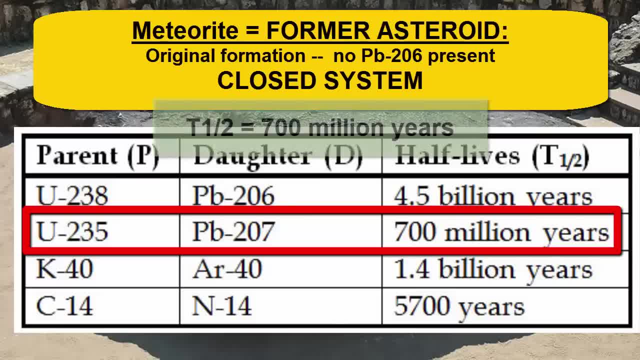 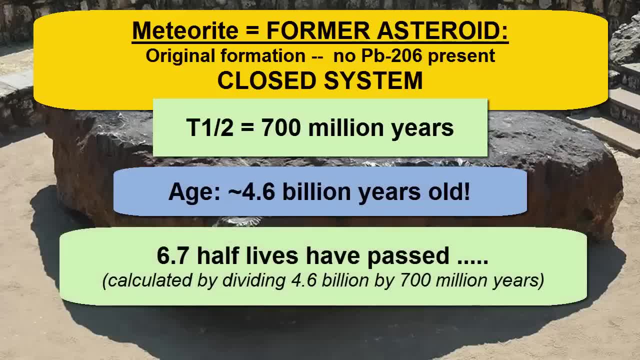 Remember, the half-life for uranium-235 to lead-207 is 700 million years. For something that is 4.6 billion years old, that means it would have passed through 6.7 half-lives. Let's look at what that means for the ratio. 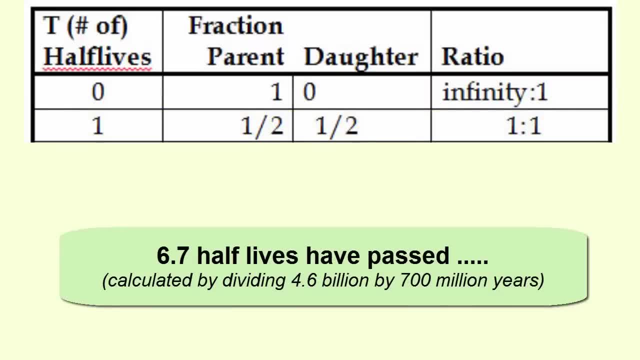 One half-life gives a ratio of one half-parent to one half-daughter, or 1 to 1.. Two half-lives have the parent again, so we have a ratio of a quarter-parent to three-quarters-daughter, or 1 to 3.. 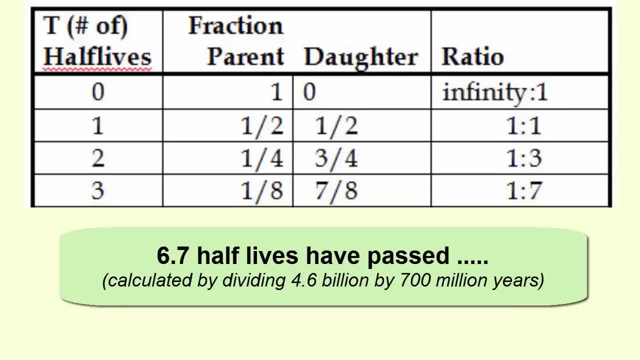 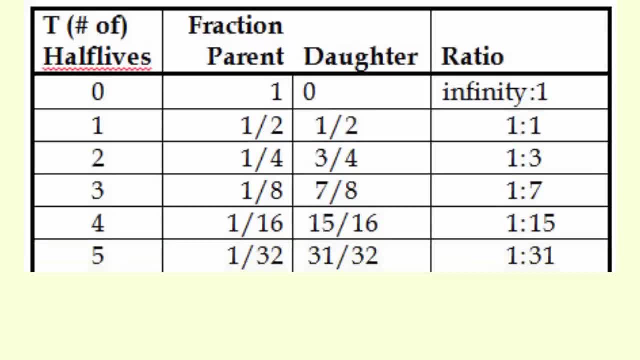 Three half-lives: one-eighth to seven-eighths, or 1 to 7.. Four half-lives: one-sixteenth to fifteen-sixteenths, or 1 to 15.. Five half-lives: one-thirty-second to thirty-one thirty-seconds, or 1 to 31.. 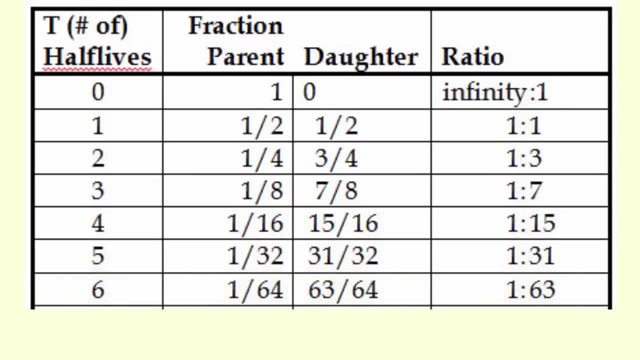 Six half-lives, one over sixty-four to sixty-three over sixty-four, or a ratio of one to sixty-three And seven half-lives is one over a hundred-and-twenty-eight parent to one-hundred-and-twenty-seven one-hundred-and-twenty-eighths daughter. 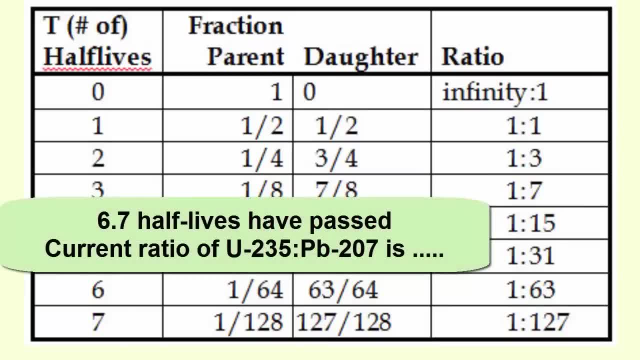 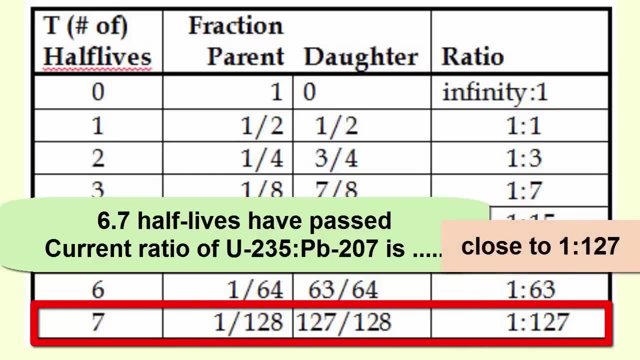 or one to one-hundred-and-twenty-eight. So the ratio we'd expect for something that had experienced 6.7 half-lives is somewhere close to 1 to 127, close to seven half-lives To be more precise. we use this equation: 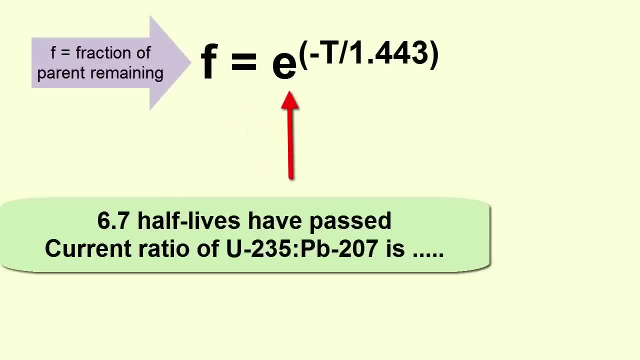 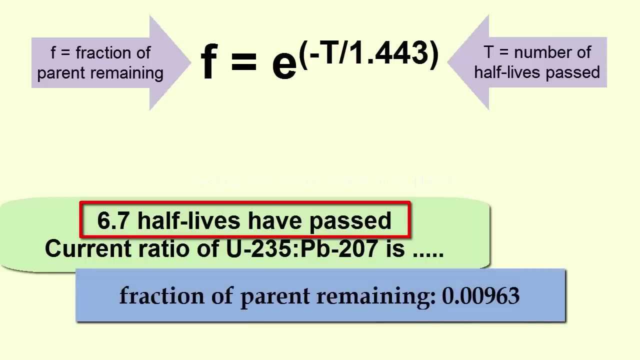 The fraction of parent remaining equals e to the power of minus t divided by 1.443, where t is the number of half-lives passed. Since t is 6.7,, that means the fraction of parent remaining is 0.00963..